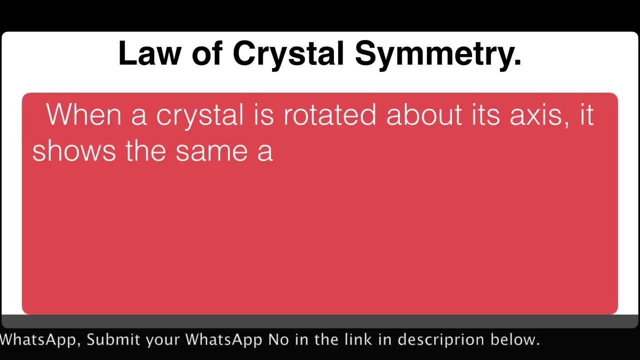 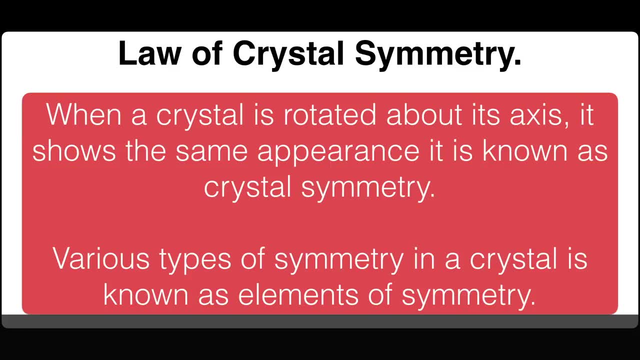 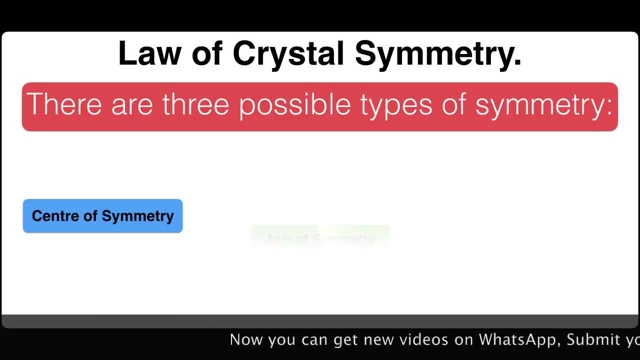 When a crystal is rotated about its axis, it shows the same appearance. It is known as crystal symmetry. Various types of symmetry in a crystal is known as elements of symmetry. There are three possible types of symmetries: Center of symmetry, axis of symmetry, plane of symmetry. So let's talk about the center of symmetry. 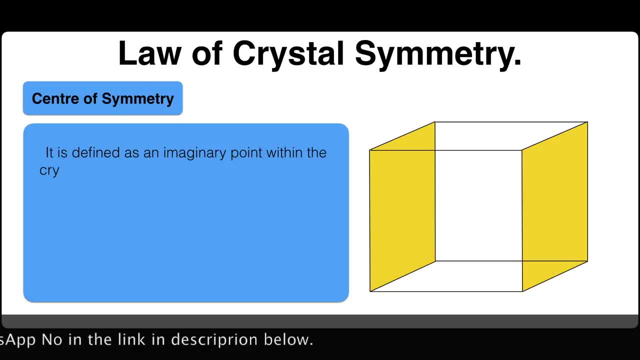 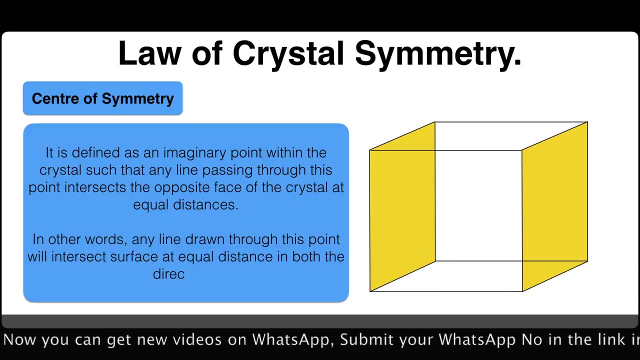 It is defined as the imaginary point within the crystal, such that any line passing through this point intercepts the opposite faces of the crystal at equal distances. In other words, any line drawn through this point will intersect surface at equal distance in both the directions. 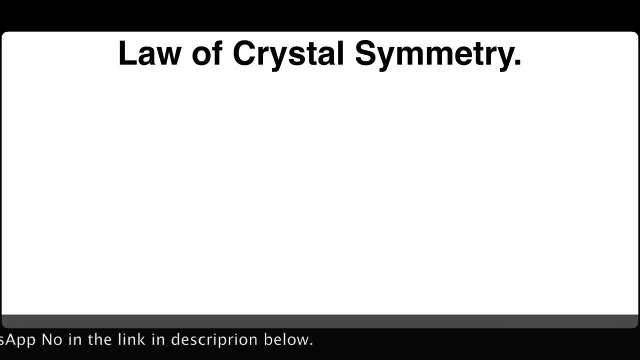 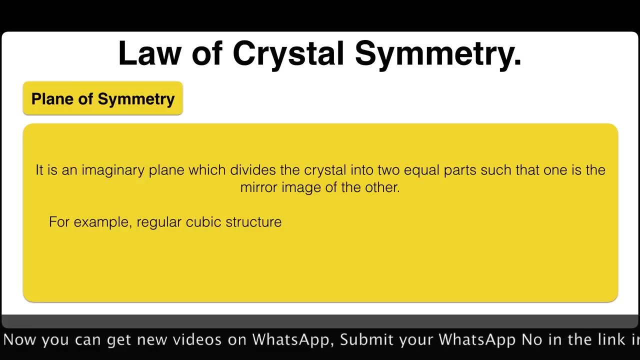 The plane of symmetry. It is an imaginary plane which divides the crystal into two equal parts, such that one is the mirror image of the other. For example, regular cubic structure can have nine plane of symmetry. Three planes of symmetry are parallel to the cube faces and six diagonal planes. 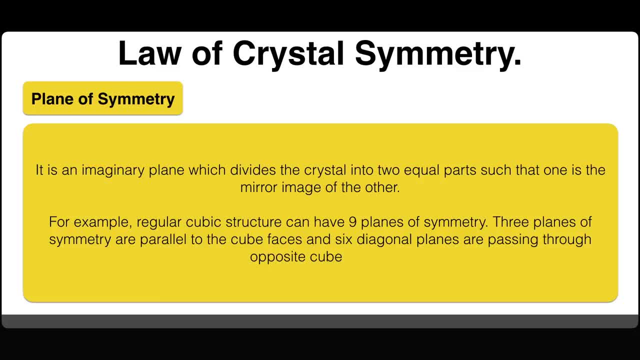 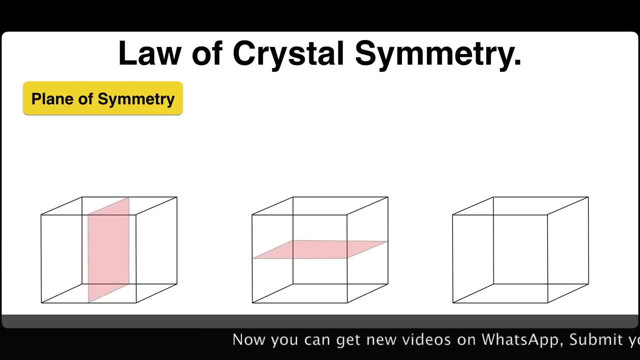 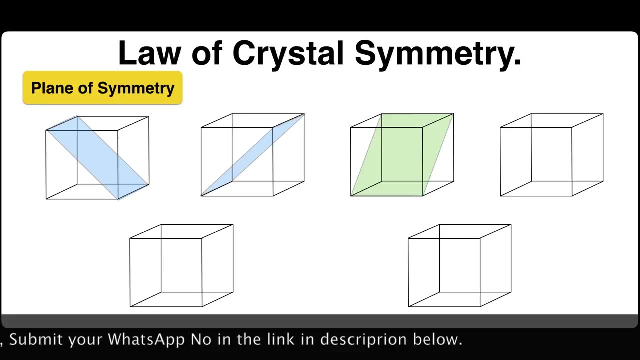 are passing through opposite cubic edges. The plane of symmetry is a plane of symmetry. These are parallel planes of symmetry. These are diagonal planes of symmetry, Axes of symmetry. Axes of symmetry is a line about which the crystal may be rotated such that it 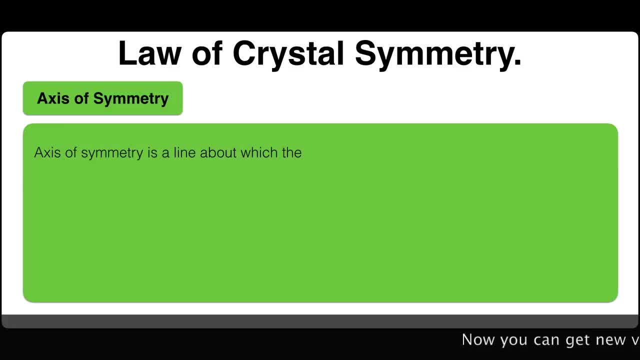 presents the same appearance more than once during the complete revolution of the world. There are manyvy things that can occur withangi monitoring the crystals and those which are supported through 360 degrees, If a crystal presents the same appearance n times in one complete revolution. 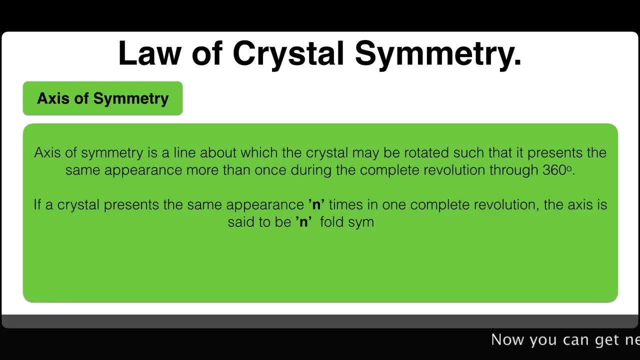 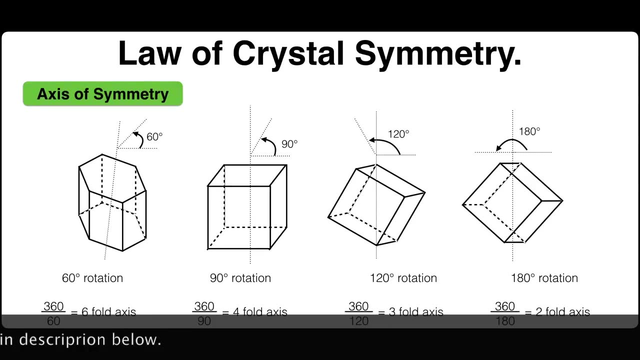 the axis is said to be n-fold symmetry. For example, the cubic crystal of sodium chloride has 13 axis of symmetry, out of which 4 are 3-fold, 3 are 4-fold and 6 are 2-fold. Following are the examples: when hexagonal structure is rotated through 60 degrees, it